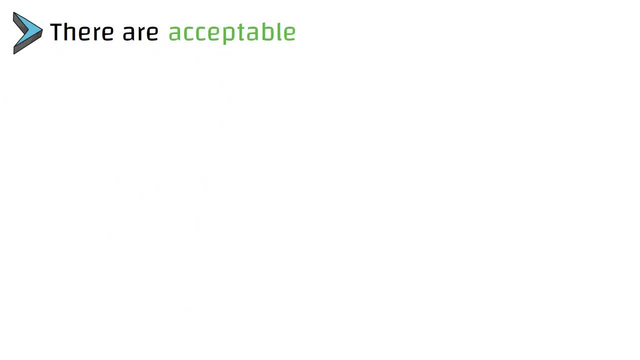 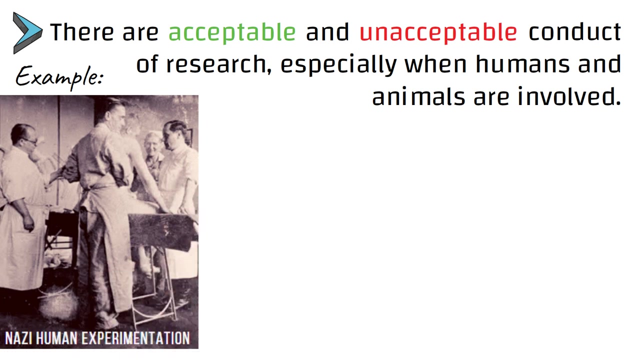 As we can see, there are acceptable and unacceptable conduct of research, especially when humans and animals are involved. Needless to say, research misconduct can lead to dire consequences if ignored. Just consider, for example, the famous Nazi human experimentation. As is well known, the Nazi human experimentation was a series of medical experiments. 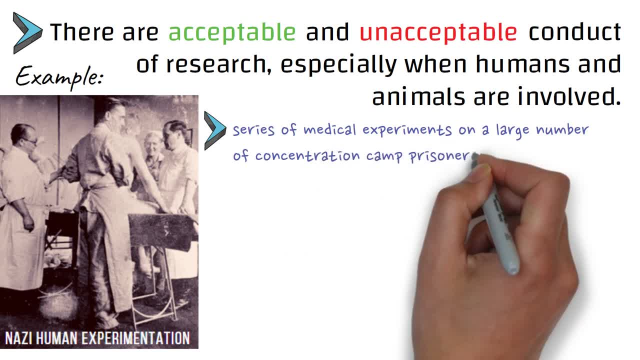 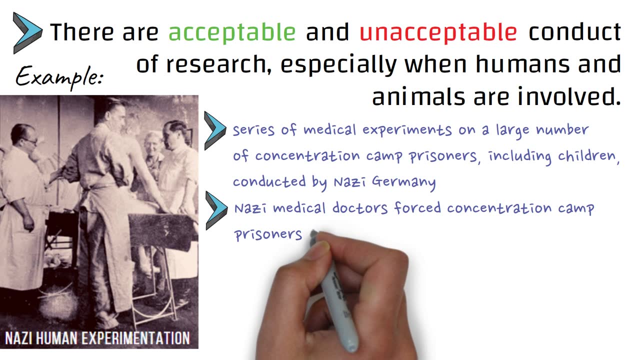 on a large number of concentration camp prisoners, including children, conducted by Nazi Germany. As is well known, during the Nazi regime in Germany, Nazi medical doctors forced concentration camp prisoners to participate in the experiment. In fact, the prisoners did not willingly volunteer. 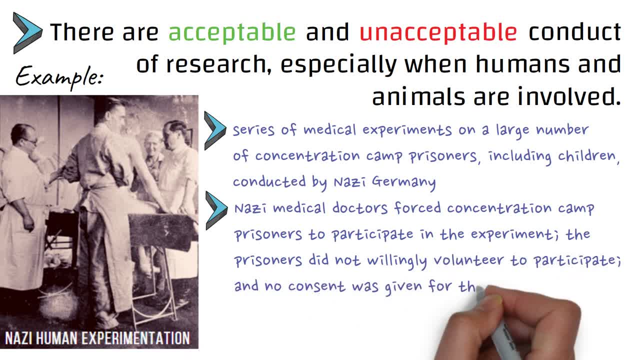 to participate in the experiment. In fact, the prisoners did not willingly volunteer to participate in the experiment and no consent was given for the procedures. As records show, the experiments had resulted in trauma, disfigurement, permanent disability and death. 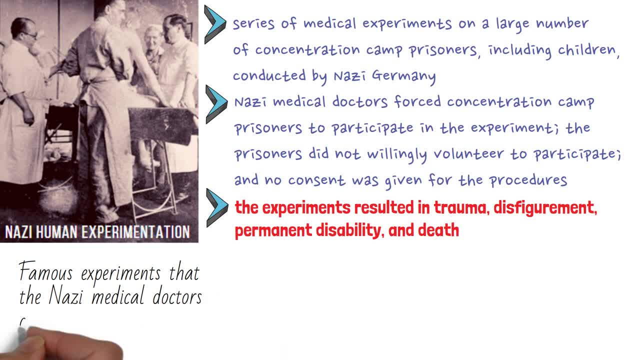 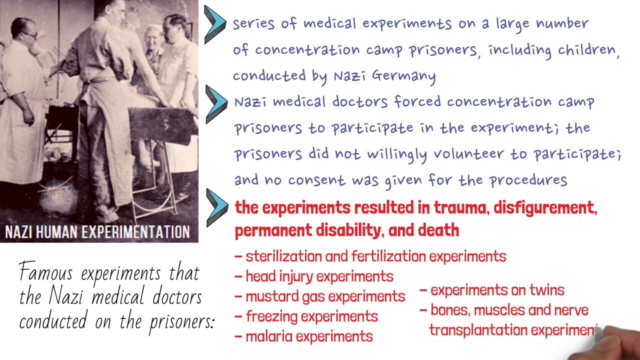 Some of the famous experiments that the Nazi medical doctors conducted in the prisoners include sterilization and fertilization experiments, head injury experiments, mustard gas experiments, freezing experiments, malaria experiments, experiments on twins and bones, muscles and nerve transplantation experiments. Now here are some ethical principles that guide research. 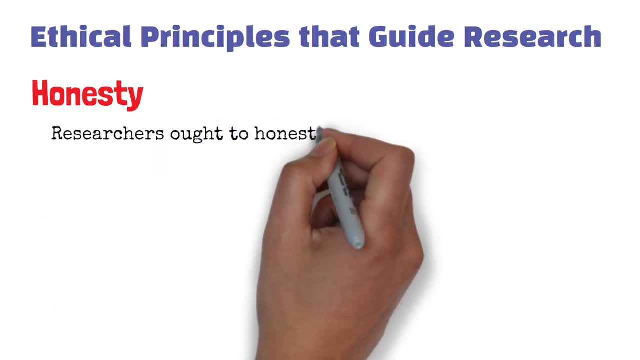 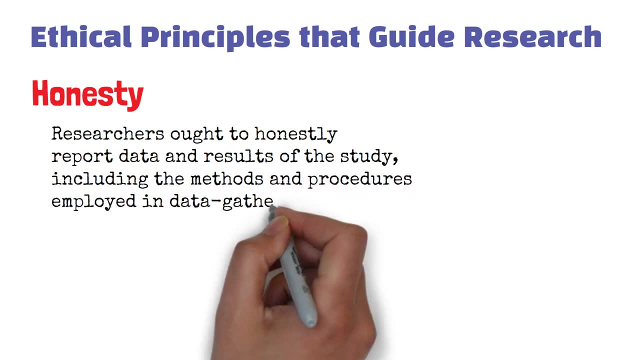 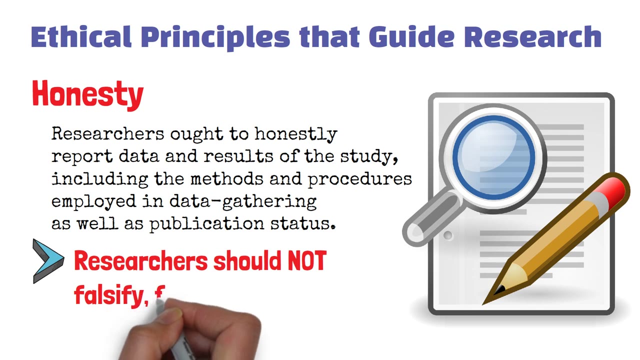 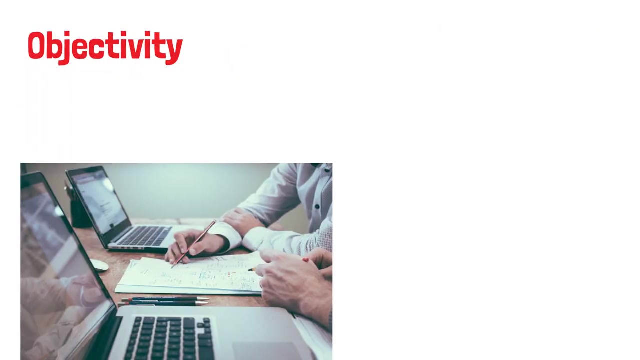 Honesty: Researchers ought to honestly report data and results of the study, including the methods and procedures employed in data gathering, as well as publication status. Thus, researchers should not falsify, fabricate and misrepresent data and results. Objectivity: Researchers should uphold objectivity and scientific rigor at all times. 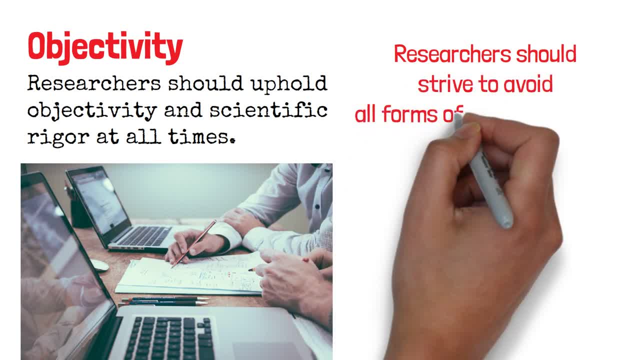 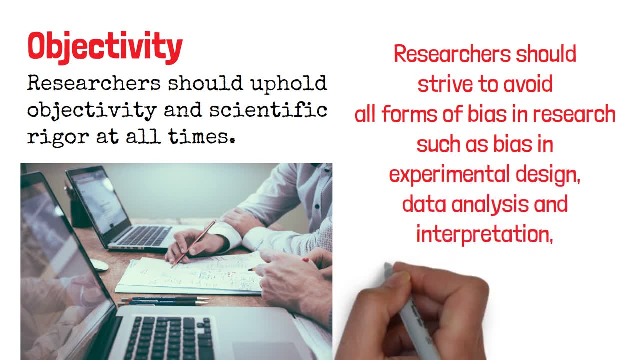 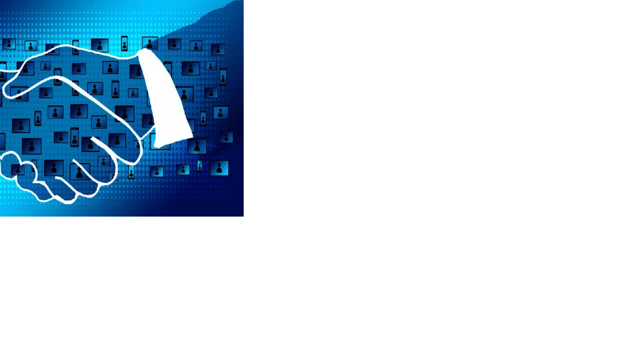 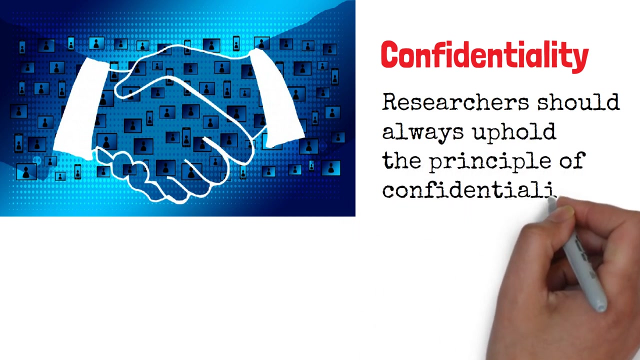 Thus, researchers should strive to avoid all forms of bias in research, such as bias in experimental design, data analysis, bias in interpretation, peer-review process, grant writing and other facets of research Confidentiality. Researchers should always uphold the principle of confidentiality. 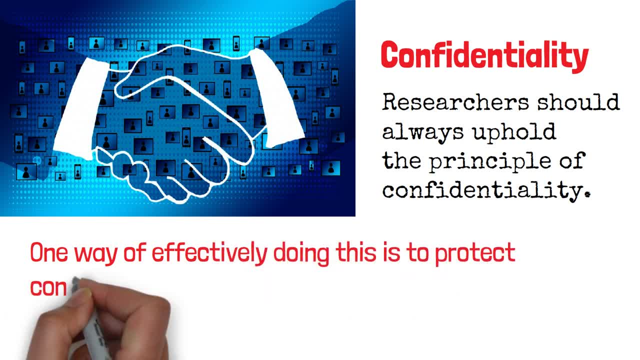 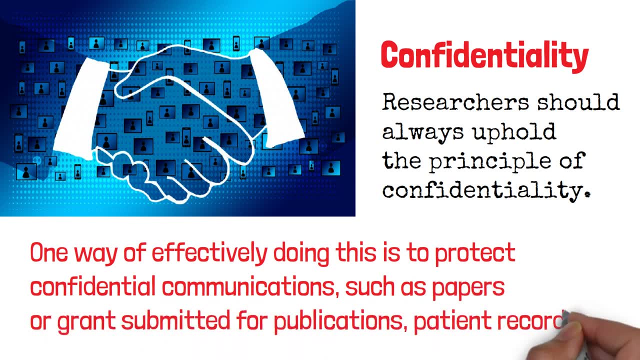 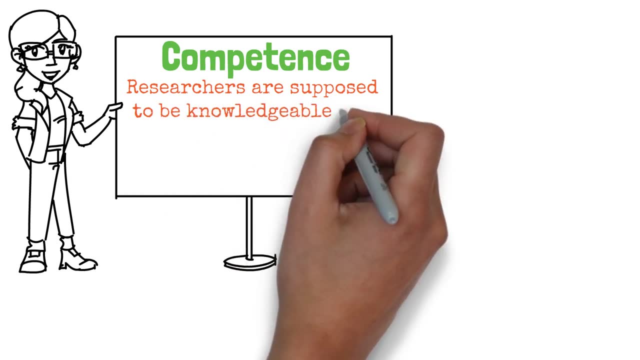 One way of effectively doing this is to protect confidential communications such as papers or grants submitted for publications, patient records and the like. Competence, Competence, Competence. Researchers are supposed to be knowledgeable and experts in their own discipline or field of specialization. 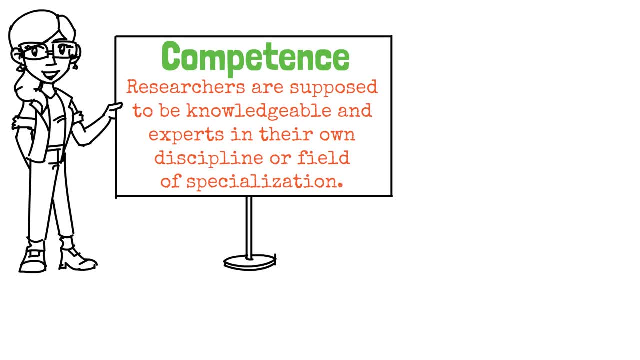 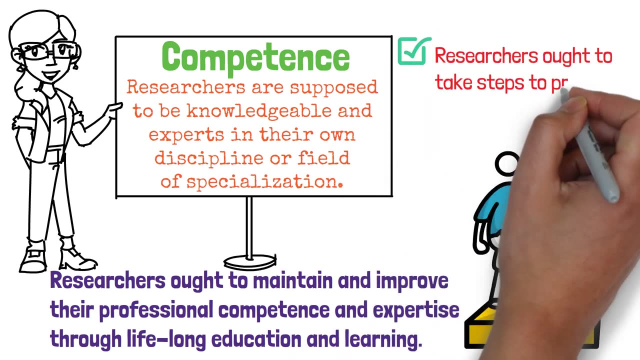 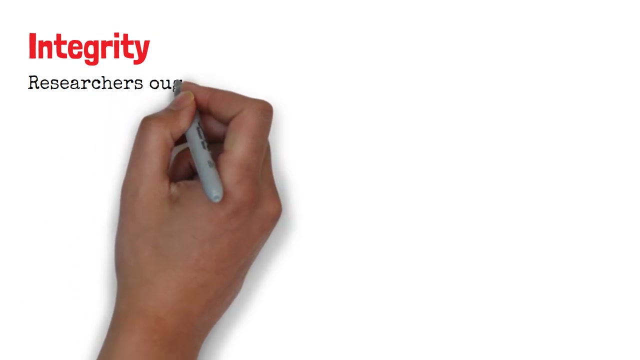 In short, researchers should be competent scholars. Thus, they ought to maintain and improve their professional competence and expertise through lifelong education and learning. More importantly, they ought to take steps to promote competence in science. Integrity: Researchers ought to keep their promises and honor agreements. 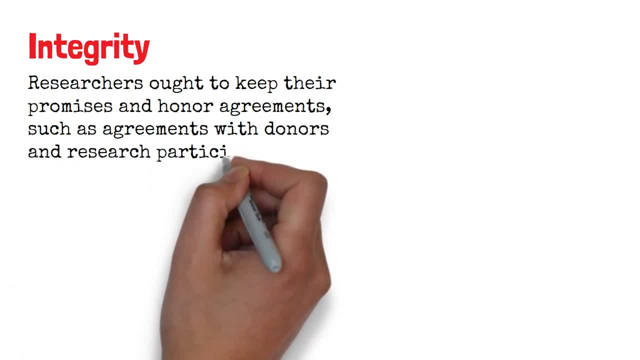 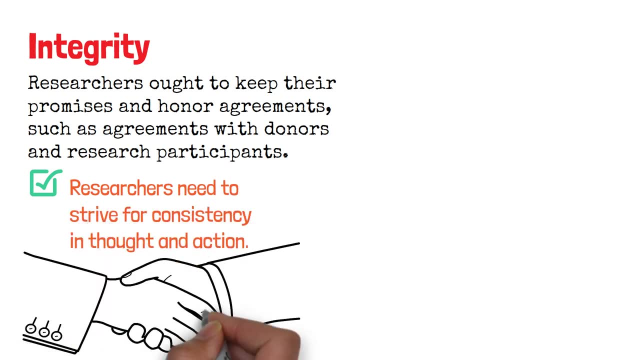 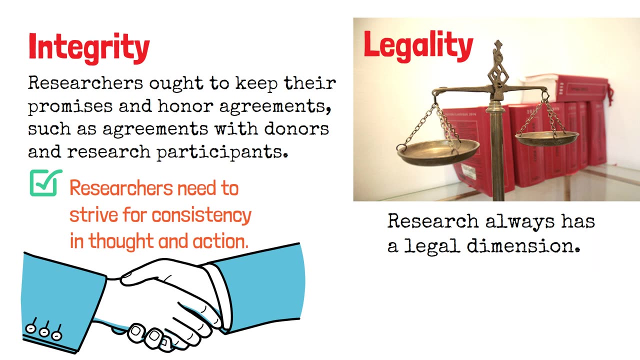 such as agreements with donors and research participants. Thus, researchers need to strive for consistency in thought and action. Legality: Research always has a legal dimension. Thus researchers ought to obey laws and relevant institutional laws, Maturity and openness. Knowledge is supposed to be free. 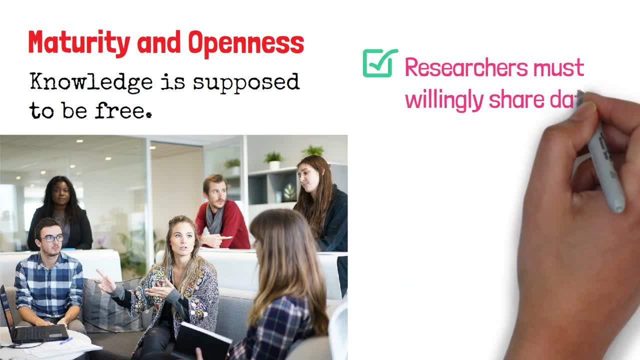 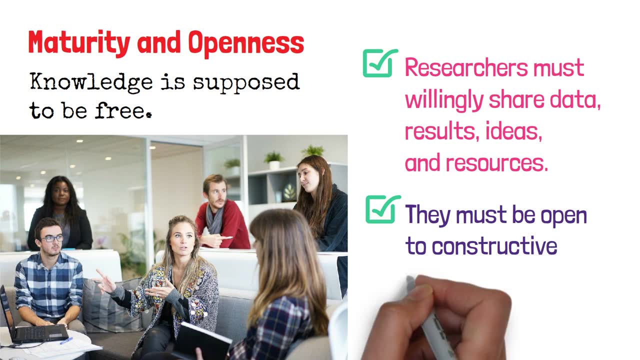 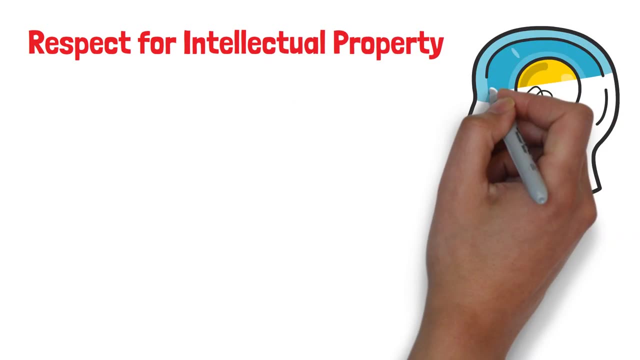 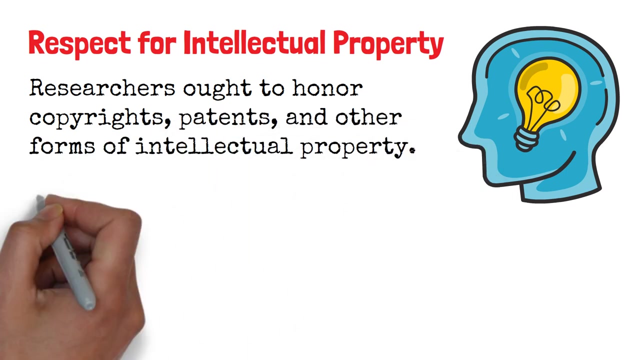 Hence, researchers must willingly share data, results, ideas and resources. They must also be open to constructive criticisms and new ideas. Respect for intellectual property: Researchers ought to honor copyrights, rights, patents and other forms of intellectual property. Thus, they should not use methods. 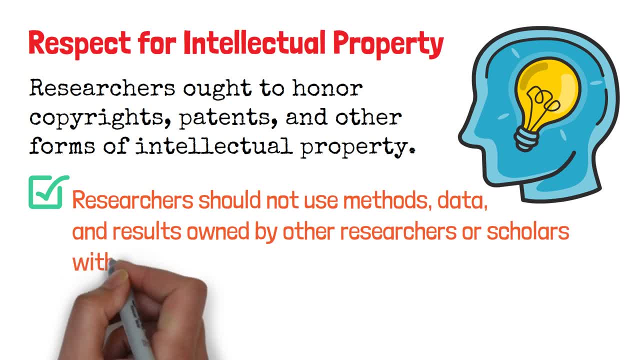 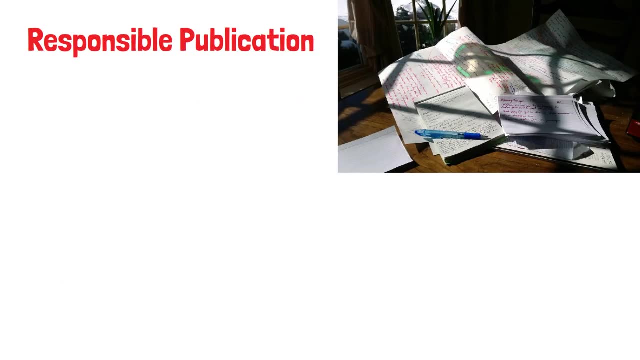 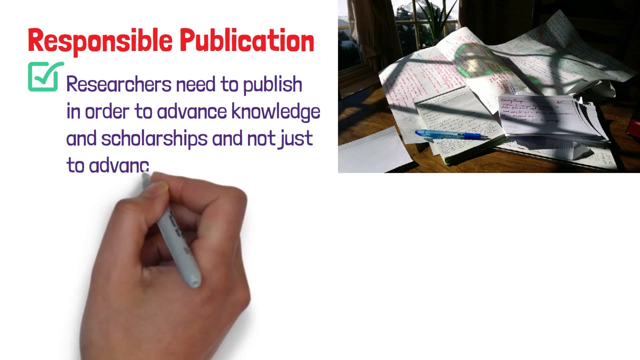 data and results owned by other researchers or scholars without permission or proper acknowledgement. More importantly, researchers should avoid plagiarism at all times. 3. Responsible publication. Researchers need to publish in order to advance knowledge and scholarships, and not just advance one's own career. They also need to avoid wasteful publication. 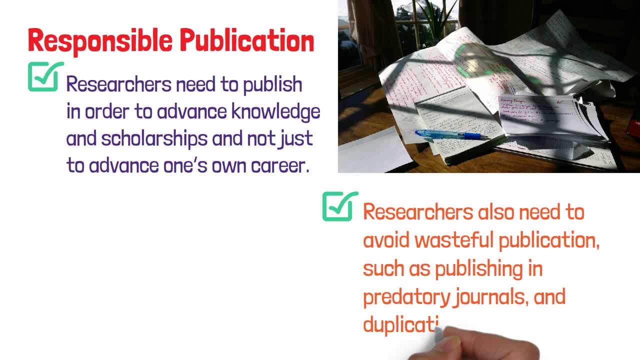 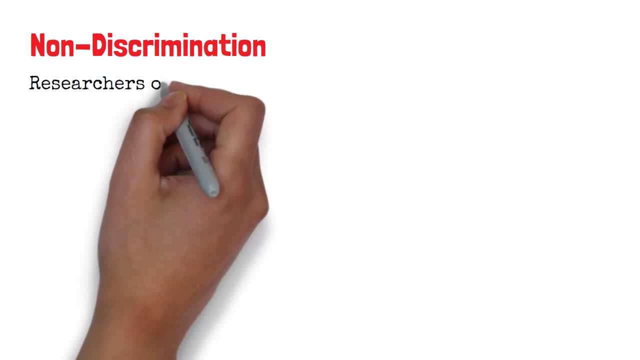 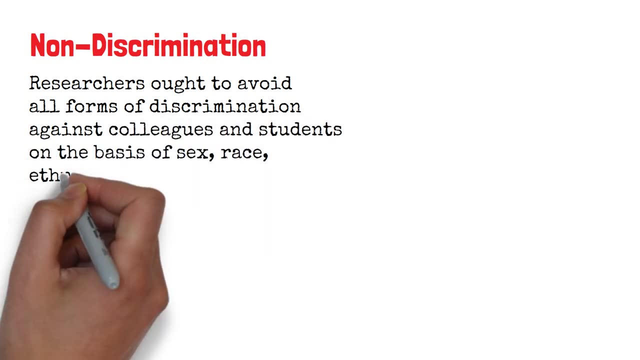 such as publishing in predatory journals and duplicative publication. 4. Non-discrimination: Researchers ought to avoid all forms of discrimination against researchers. Researchers ought to respect their colleagues and students on the basis of sex, race, ethnicity and other factors that are related to scientific competence and integrity. For this reason, 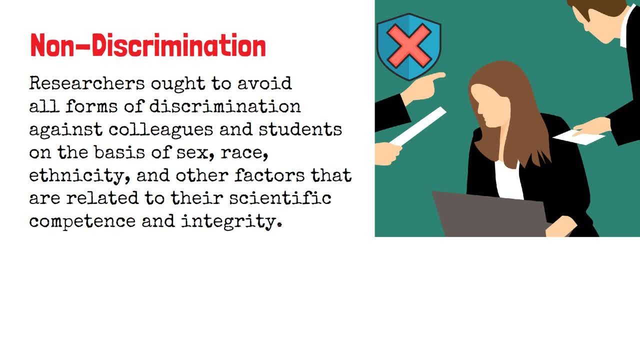 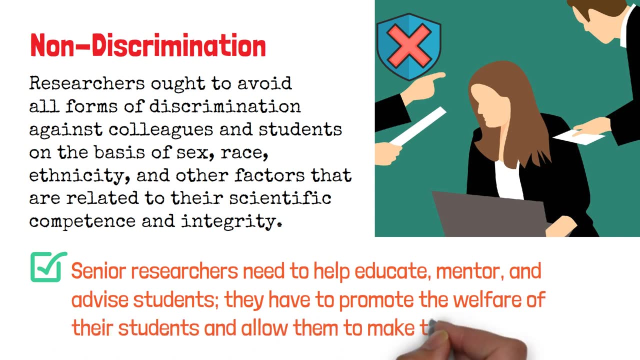 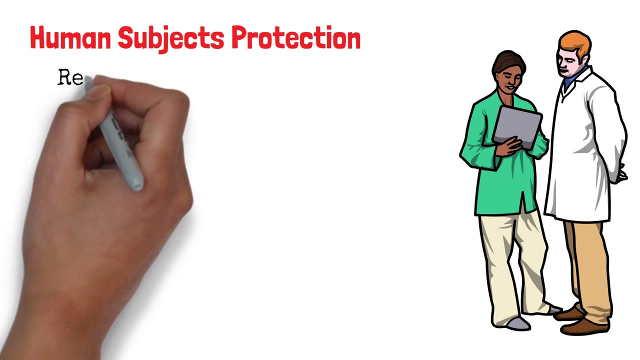 researchers ought to respect their colleagues and treat them fairly. Senior researchers also need to help educate, mentor and advise students. Senior researchers therefore have to promote the welfare of their students and allow them to do so. 5. Human subjects' protection. Researchers should respect human dignity, privacy and. 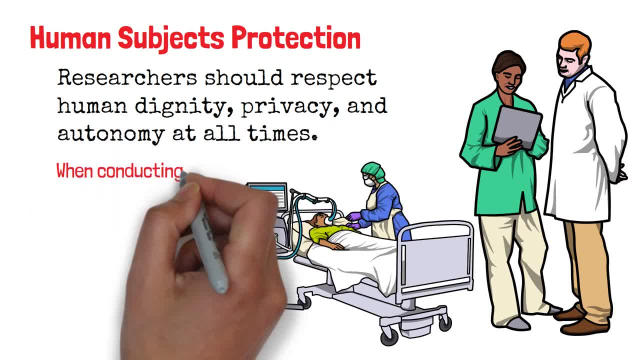 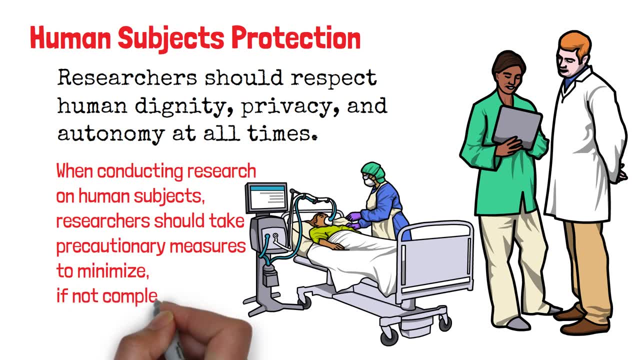 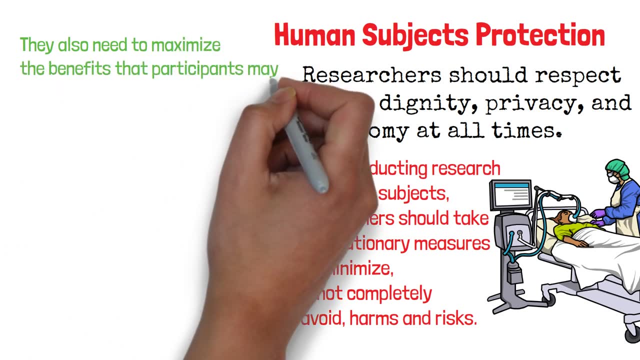 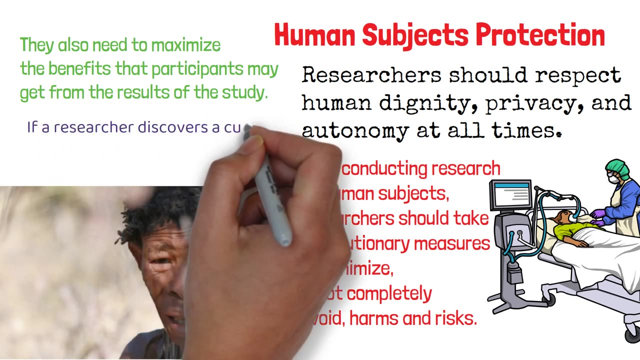 autonomy at all times. When conducting research on human subjects, researchers should take precautionary measures to minimize, if not completely avoid, harms and risks. They also need to maximize the benefits that participants may get, For instance, if a researcher discovers a cure for a particular disease through her research on. 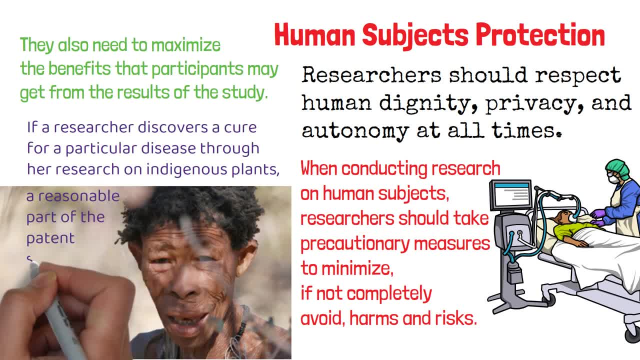 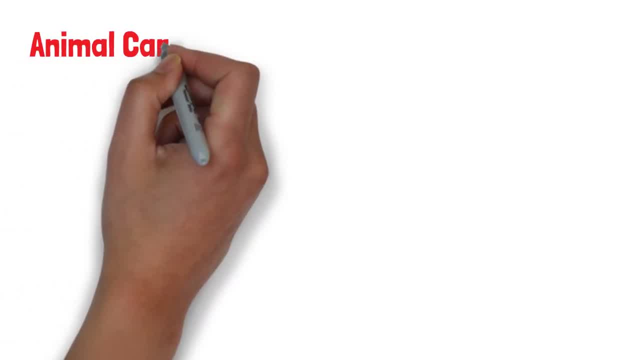 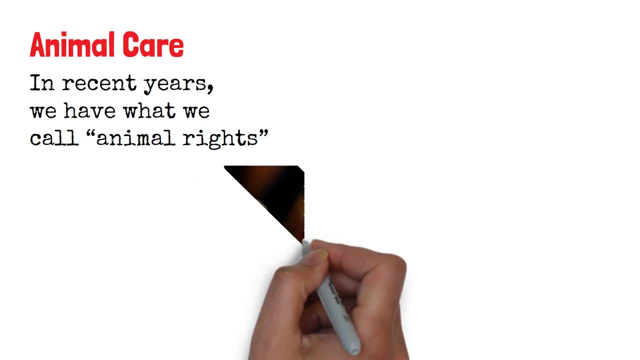 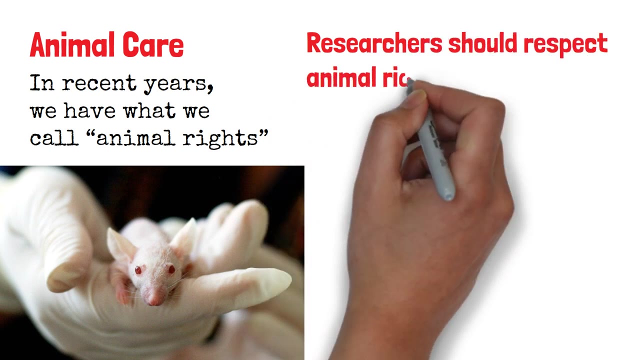 indigenous plants, a reasonable part of the patent should go to the indigenous community or communities where the plants are located. 6. Animal care. In recent years, we have what we call animal rights, thanks to the efforts of animal rights advocates. For this reason, researchers should respect animal rights at all times. As a result, 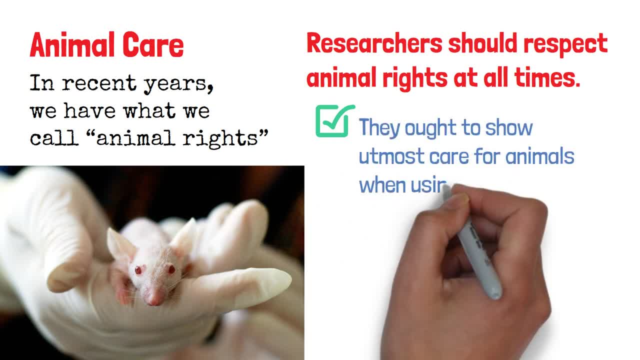 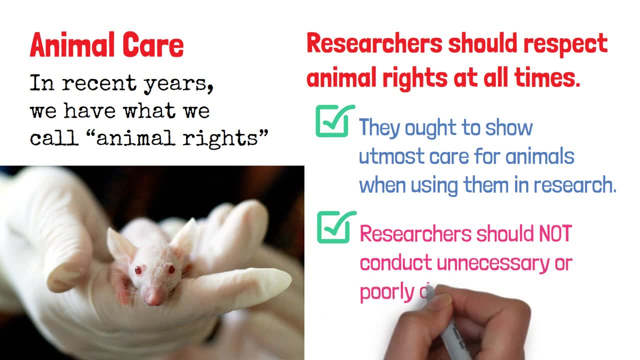 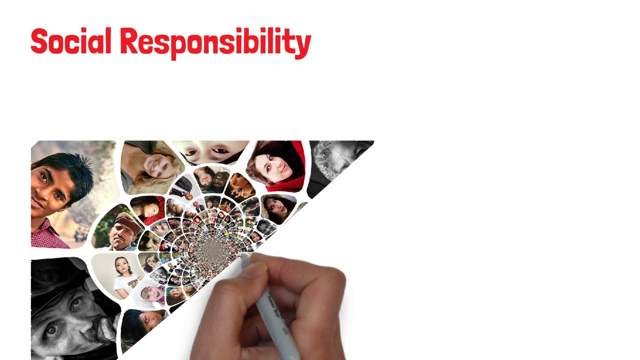 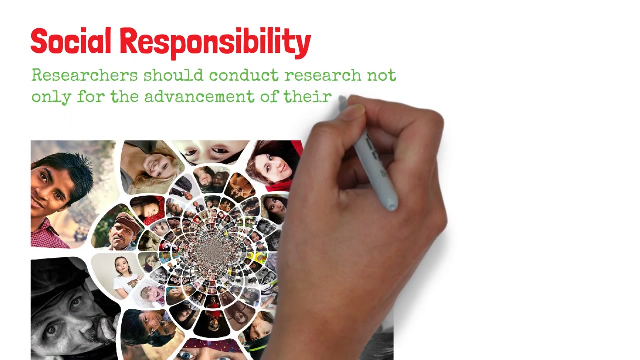 they ought to show utmost care for animals when using them in research. Researchers, therefore, should not conduct unnecessary or poorly designed animal experiments. 7. Social responsibility: As already emphasized, researchers should conduct research not only for the advancement of their own career, but for the good of society as a whole. 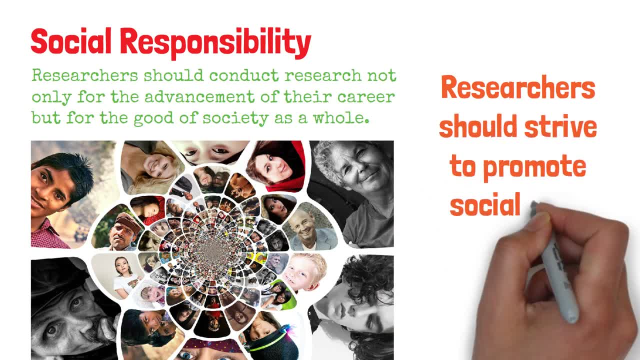 Thus, researchers should strive to promote social good and mitigate social harms.